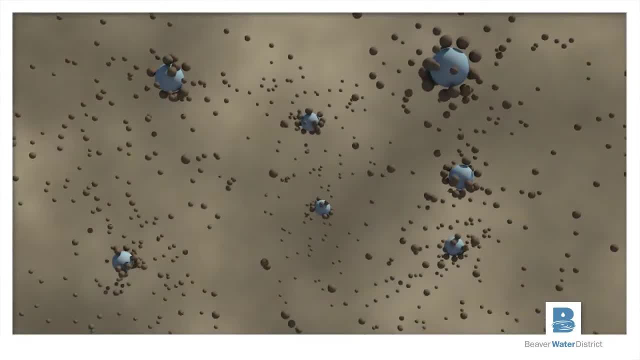 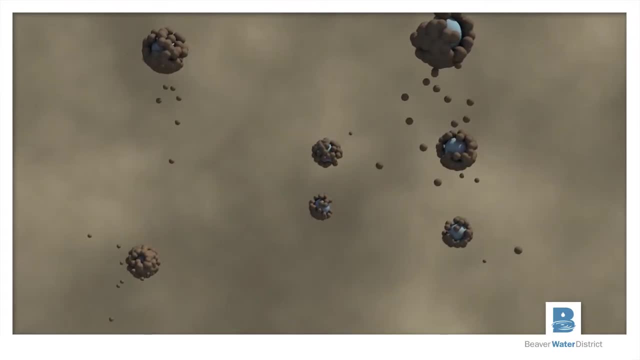 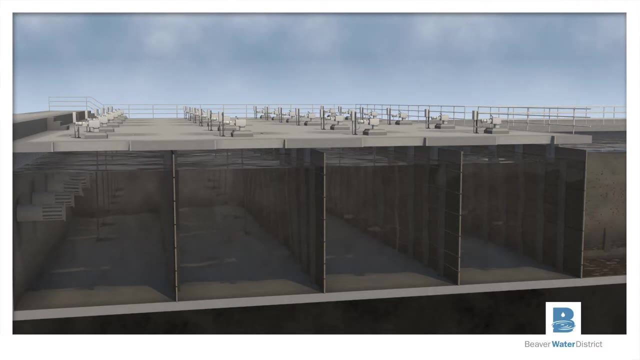 The chemical properties of the coagulant cause the dirt particles in the water to coagulate or clump together to form larger particles, known as flock. Mechanical mixers in the flocculation basins bring the smaller particles close enough together to form larger, heavier flock There. 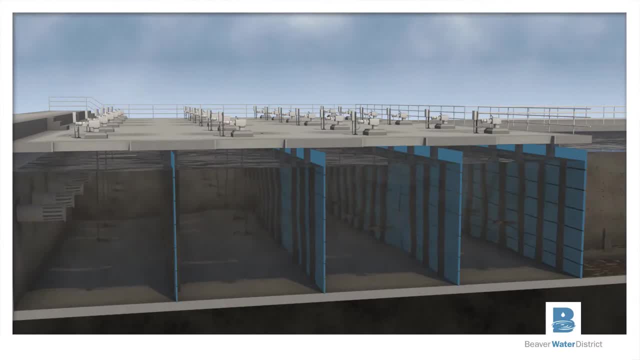 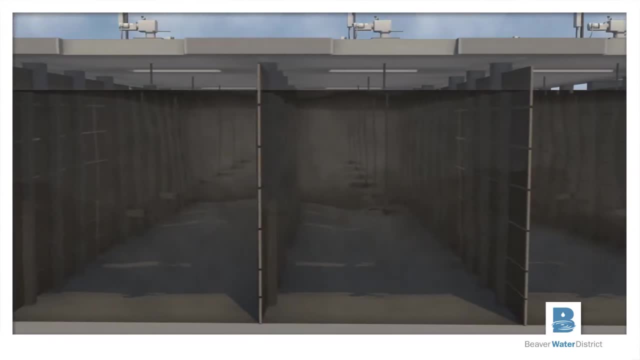 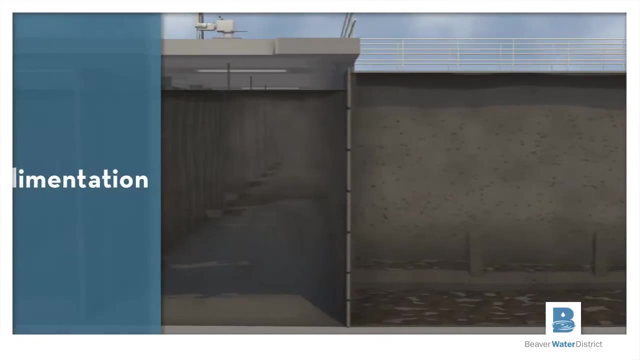 is a baffle wall separating each of the four stages in the flocculation basin. Each row of mixers is rotating at a lower speed than the previous row to prevent the delicately formed flock particles from breaking apart. Here we have enlarged and sped up the flock particles to better illustrate the sedimentation. 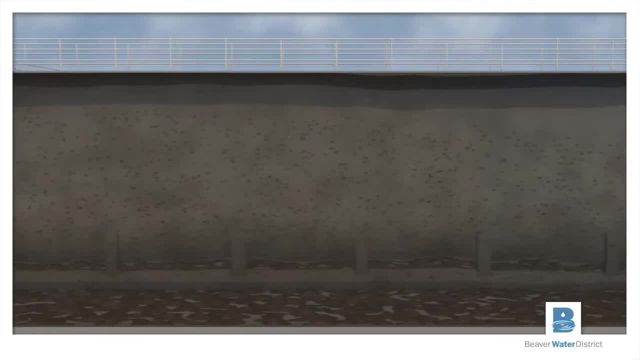 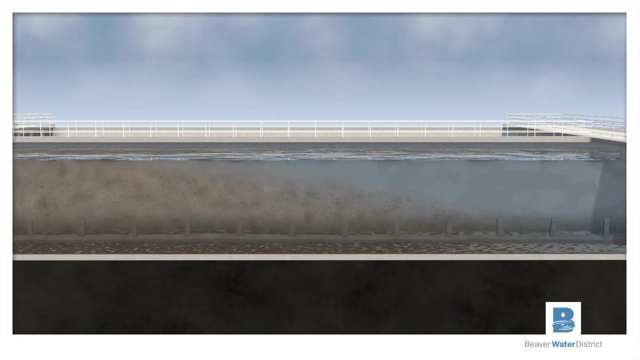 process. The larger flock particles are heavy enough to settle in the sedimentation basins It takes. It takes at least three hours for the water to move from one end of the basin to the other, which allows the very small and light flock particles to settle to the bottom of the basin. 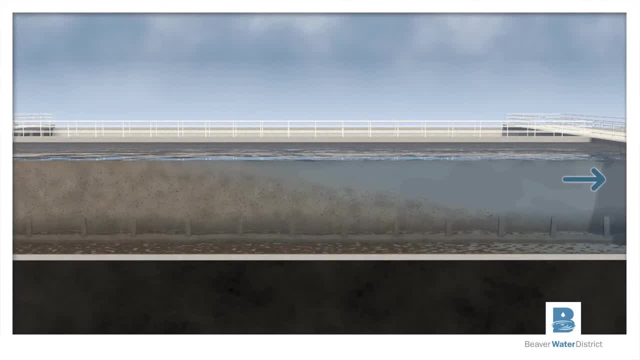 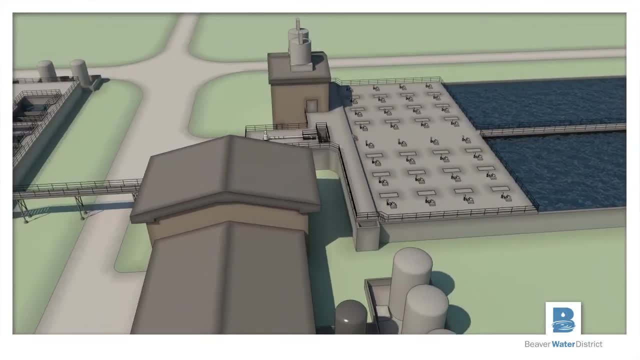 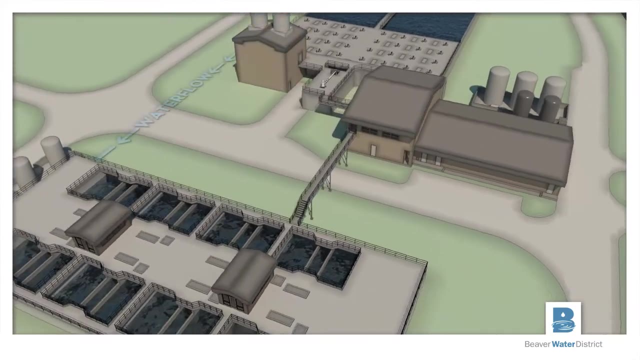 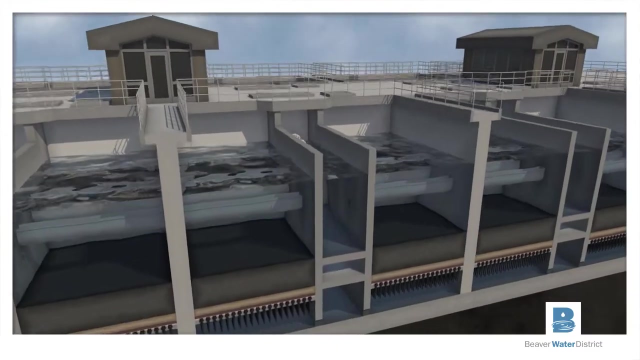 The cleaner water that flows out of the end of the sedimentation basin is called settled water. The pH of the settled water is raised by the addition of lime. Lime is delivered as a fine powder and is stored in tall silos. The settled water flows from the sedimentation basins to the filters through a buried pipe. 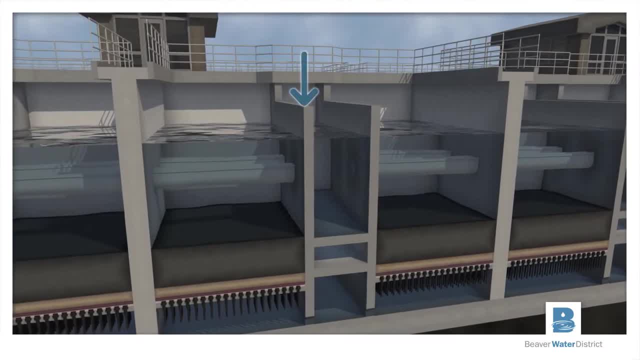 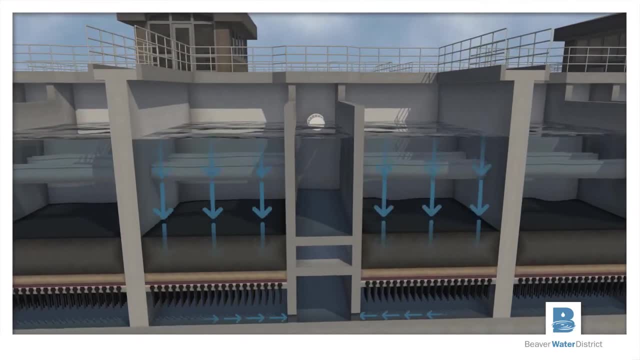 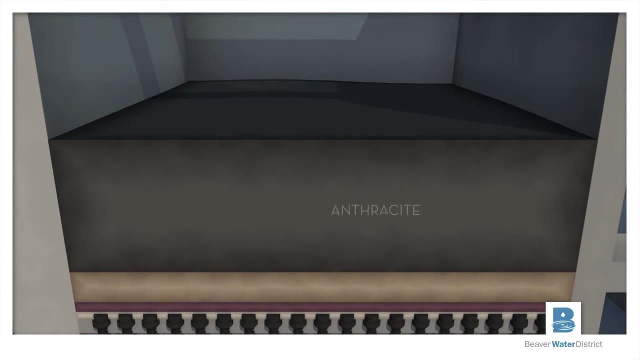 The settled water is then piped to the top of the filters, where the remaining impurities are removed. The water then simply flows by gravity from the top of the filters to the bottom through the filter media. The filter media is composed of layers of anthracite. 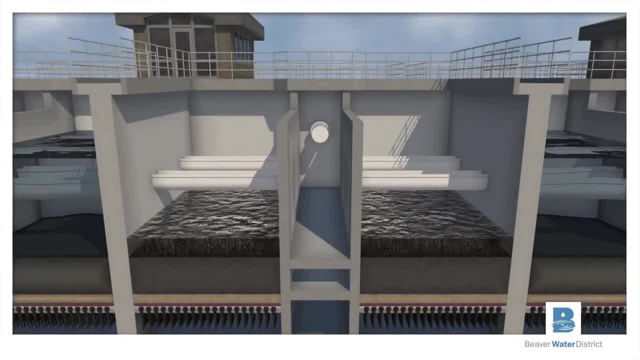 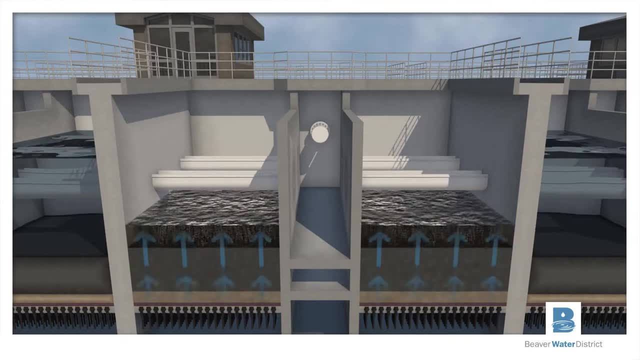 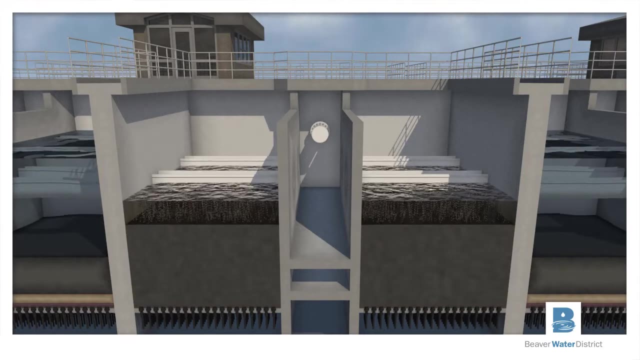 sand and garnet. The filters are periodically cleaned in a process referred to as backwashing- the forcing of water in reverse from the bottom to the top of the filters. This process tends to strongly mix the filter media, causing the dirt that was trapped in.